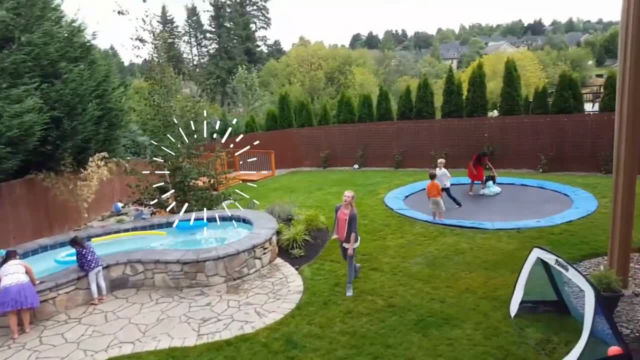 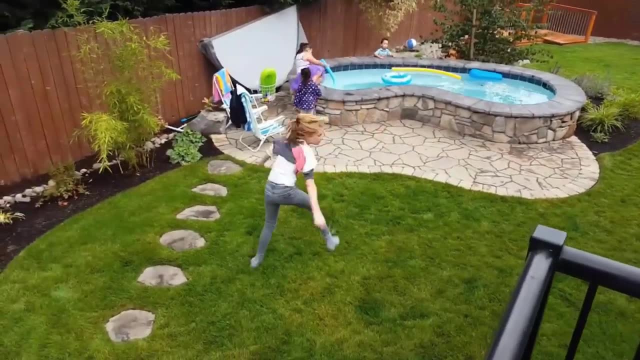 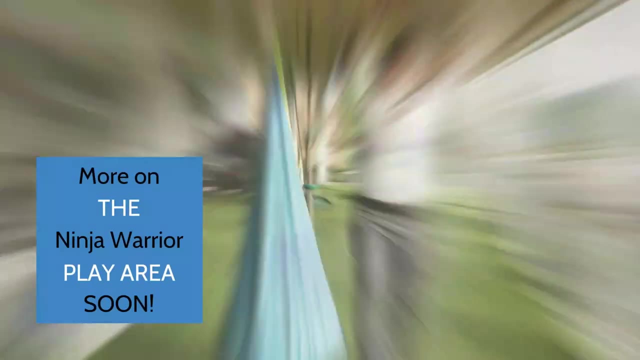 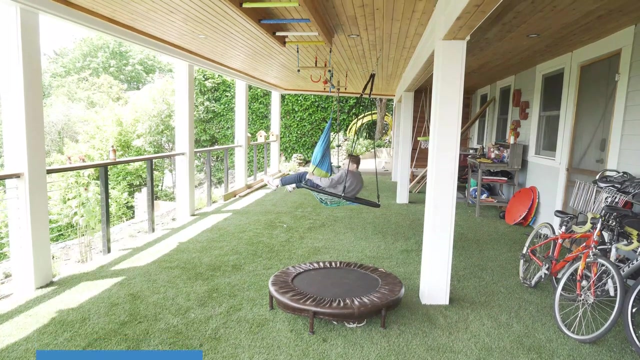 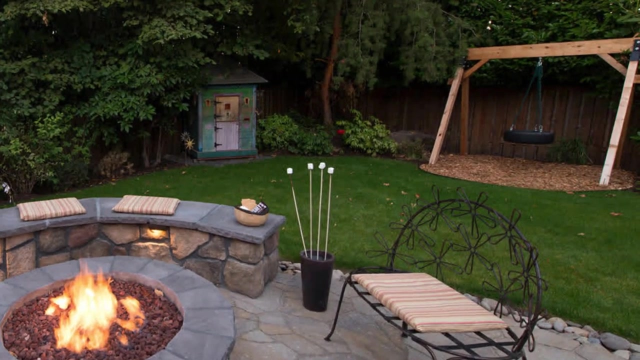 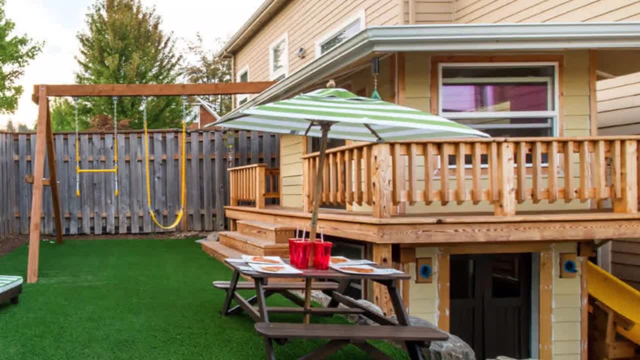 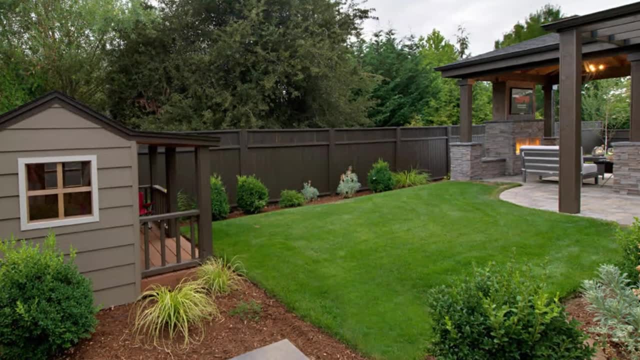 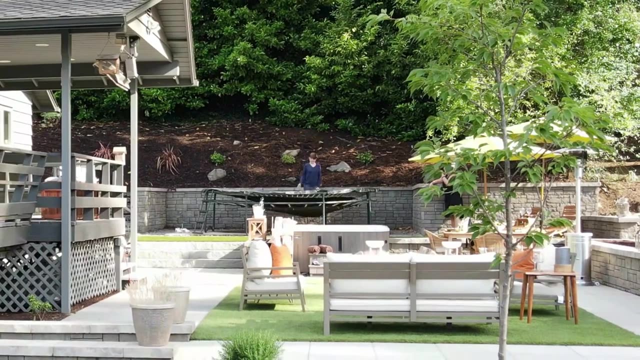 some of those in this montage. It's not just the custom playground structures which you're seeing here, It's all the different areas, different ways to get our kids outdoors having fun. It could be a trampoline area, which so many families want. It could be a camping setup. 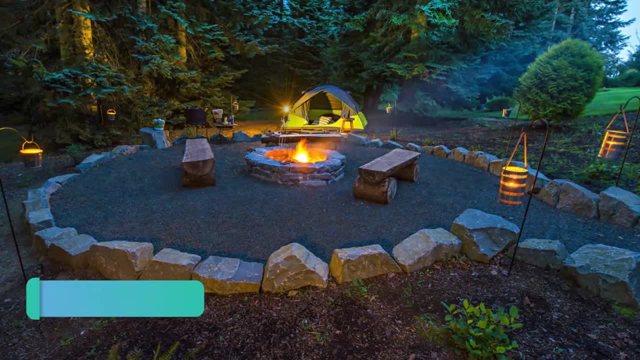 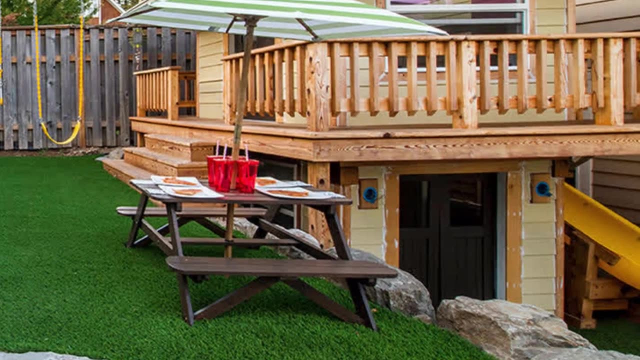 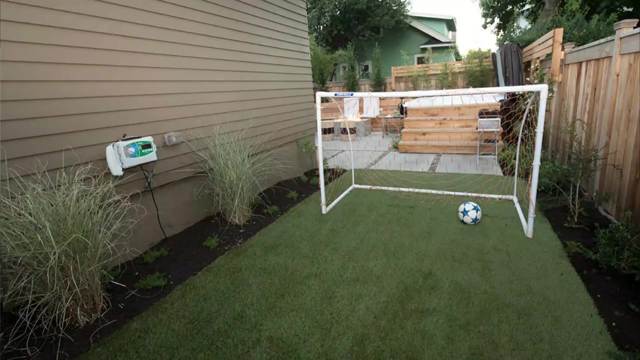 as you're seeing here. Get them outside doing the s'mores. This is a backyard. they set up a tent. you can do this. it could be a clubhouse environment where they go and they hang out and they pretend in the clubhouse. it could be a soccer side yard. it could be a basketball court. 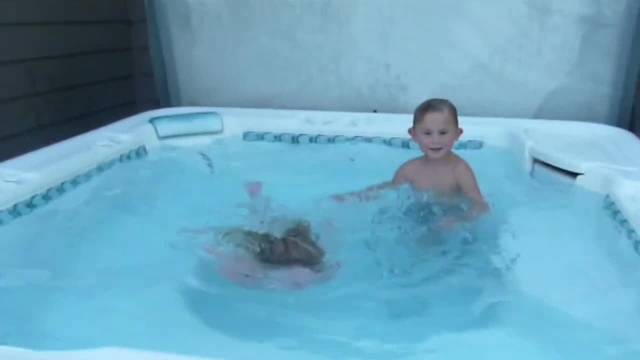 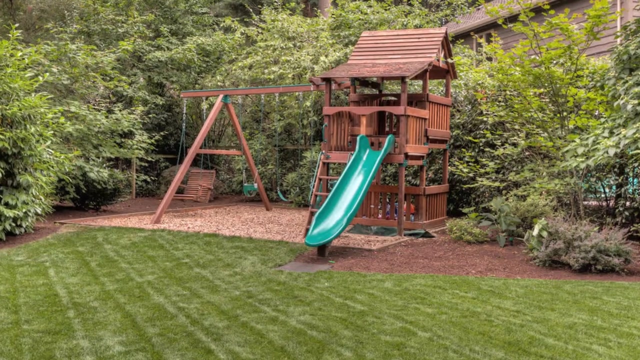 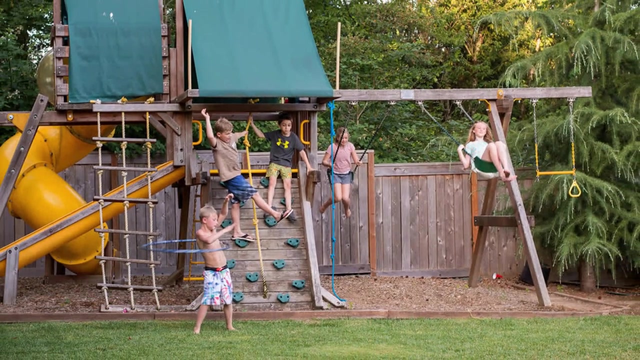 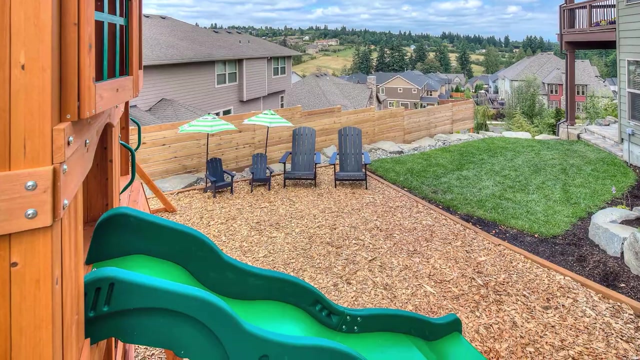 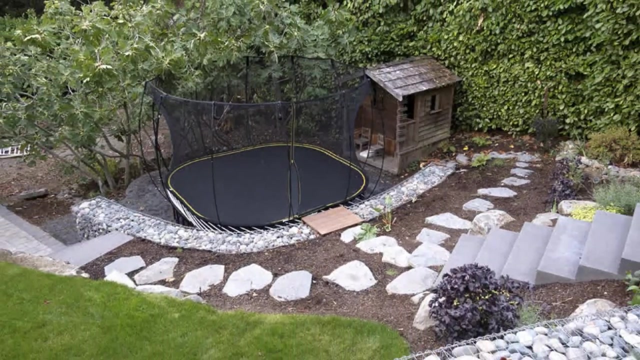 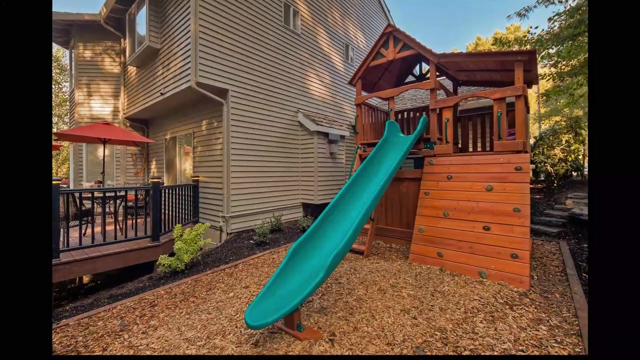 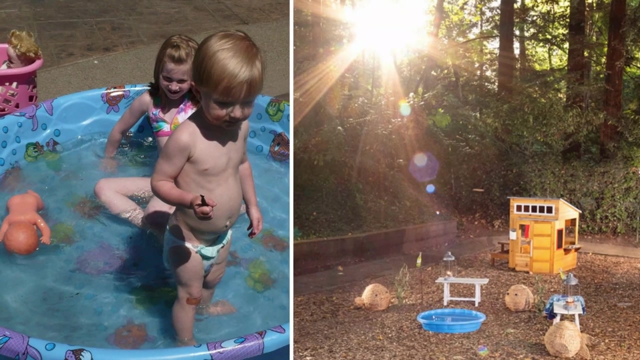 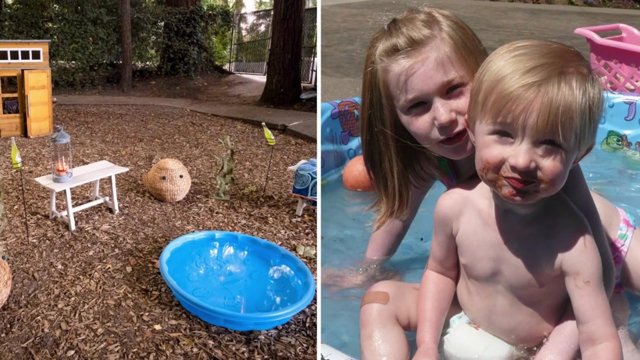 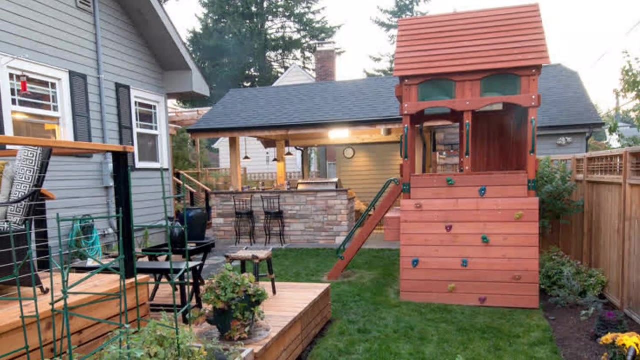 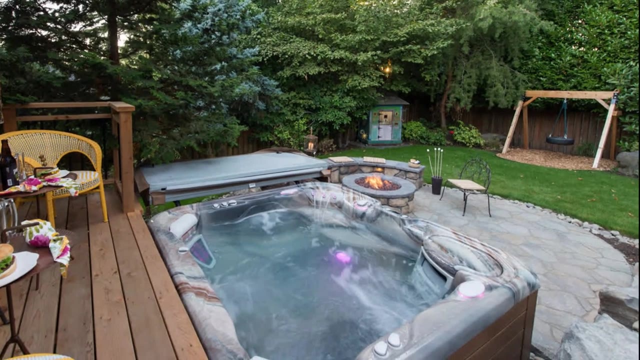 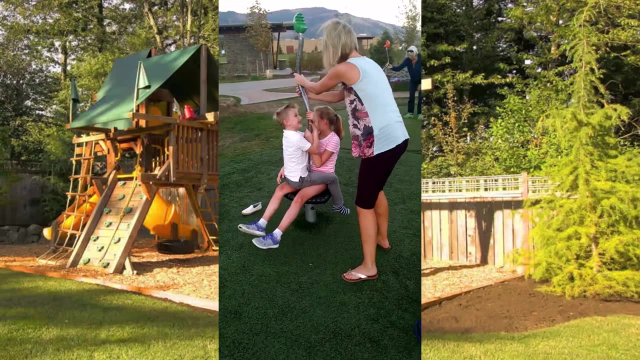 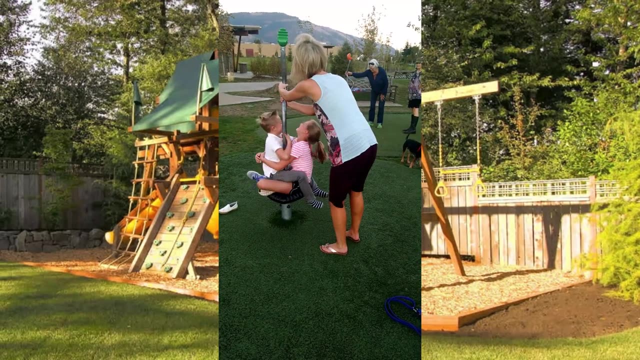 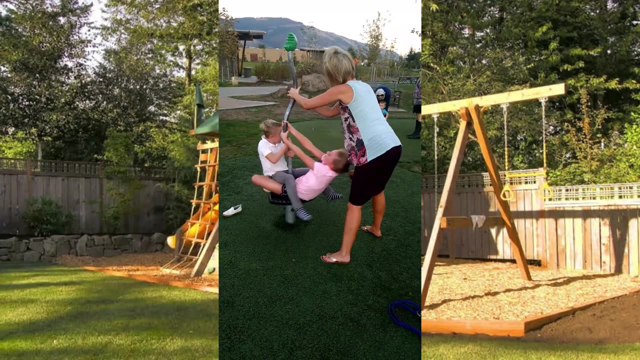 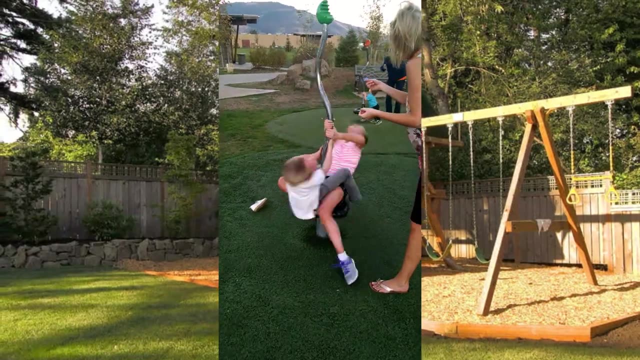 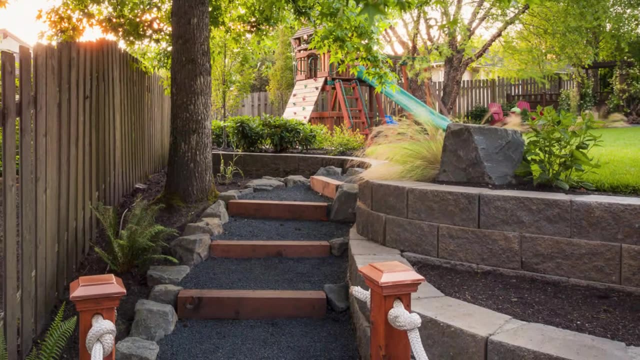 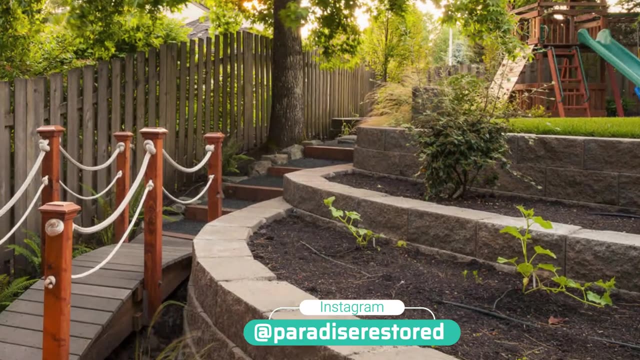 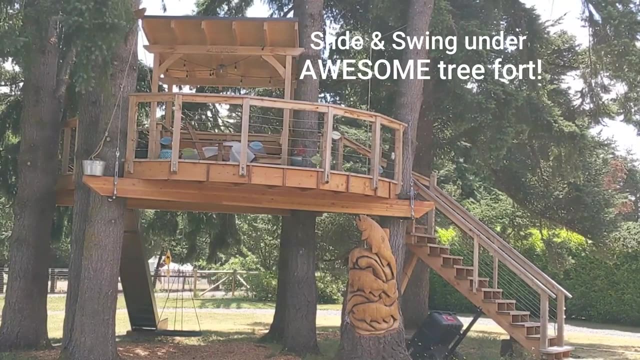 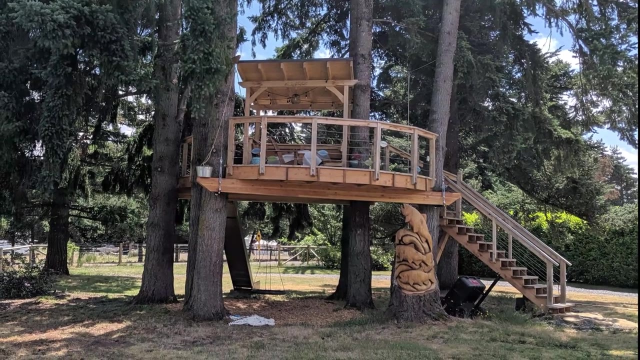 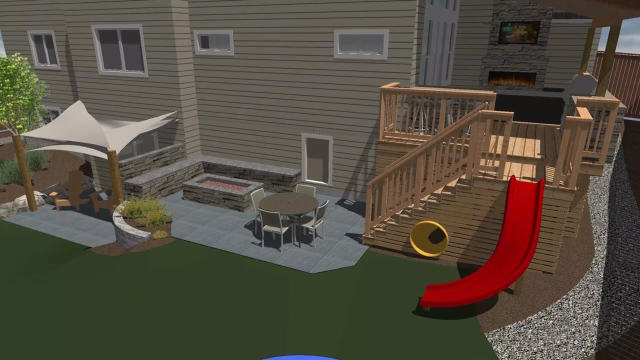 it could be a hot tub, whatever we can do to get our kids outside. that's the goal, that's what we want to accomplish and that's the ideas that I'm hoping I'm showing you in this video. you, hey, good design will help find the right spot and make sure everything. 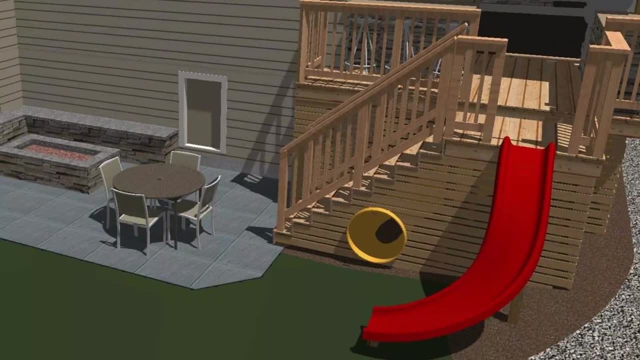 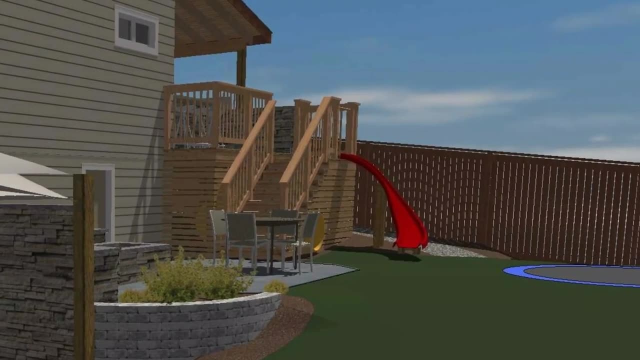 is in the right spot and make sure everything is in the right spot and make sure everything else with the landscape flows, for not only the little ones, but for the adults as well. as you can see here with the design, we installed a slide from the deck down to the synthetic lawn. so what a great. 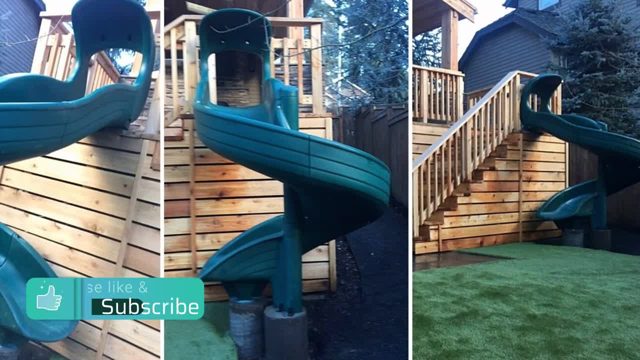 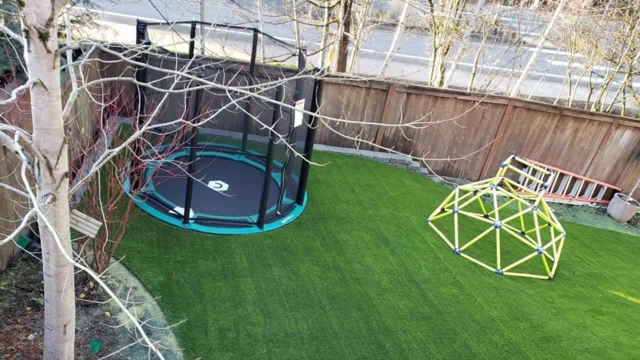 way to get down from your upper deck, then just slide on down. now, over in the synthetic lawn area, we installed a trampoline- this was built in ground- and then we did some other play structure areas. but the highlight really is the fact that we installed a trampoline and then we did some. 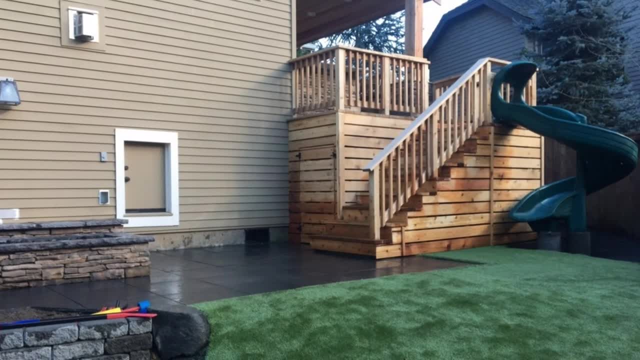 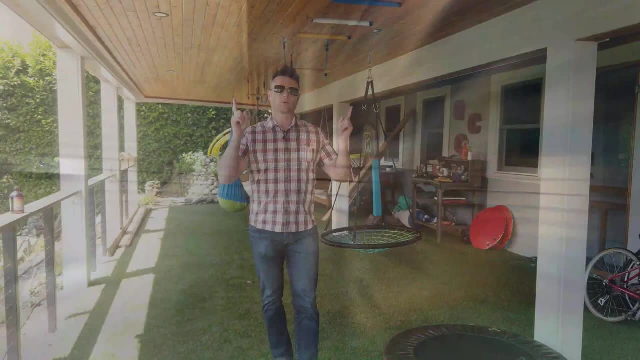 other play structure areas. but the highlight really is the fact that we installed a trampoline, the slide off of the deck and just the ability to run around in the lawn and use that trampoline. the waterproof, the deck put in the tongue of groove, put in the lighting and we put in.